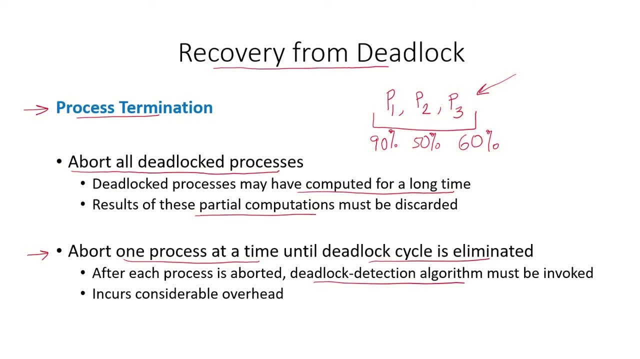 detection algorithm will be invoked to check whether the remaining processes are deadlocked or not. If the deadlock is still existing, then again another process will be chosen. So let's say first we had these three processes, P1, P2 and P3, in a deadlock. So initially the deadlock process. 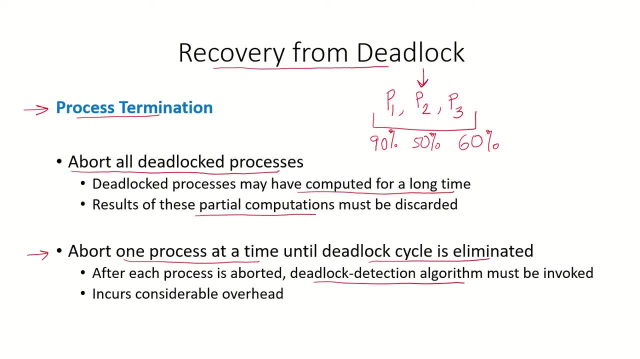 initially, let's say P2 has been chosen to be aborted. So once P2 has been aborted again, the deadlock detection algorithm will run to check whether P1 and P3 are still in a deadlocked state or not. If they are not in a deadlocked state, then it is okay, but if they are in a deadlocked state, 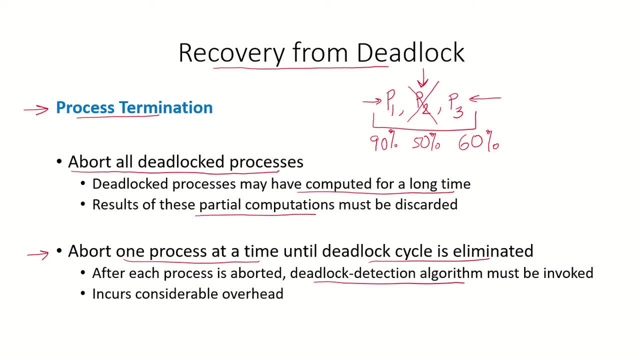 again out of these processes, P1 and P3, again one process will be chosen, and so on. Now that means that after each process is aborted, this deadlock detection algorithm has to be invoked. So this incurs considerable overhead, because every time a process is being aborted, 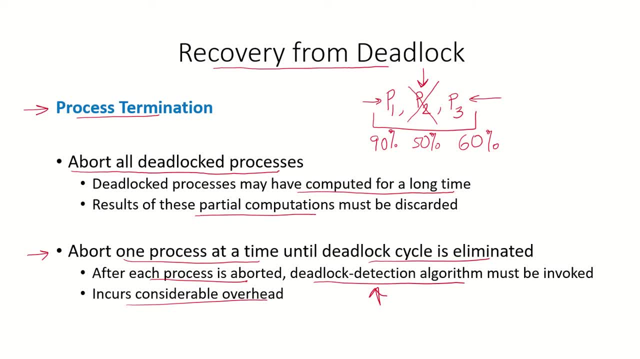 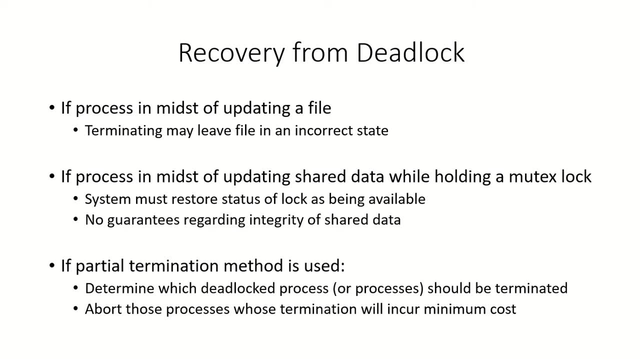 a detection algorithm has to be invoked to check for deadlock. Now, if a process is terminated? there are various situations in which a process might be terminated. There is a possibility that the process was in the middle of updating a file and now terminating that process may leave the file in an incorrect state. There is another. 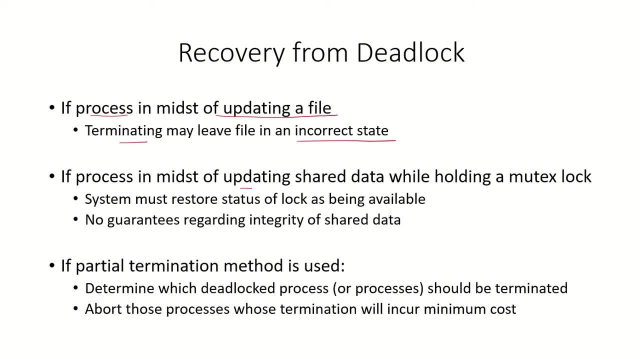 possibility that the process was in the middle of updating shared data while holding a mutex locks. So now, if this particular process is terminated, then the system must restore the status of the lock as now available and there is no guarantee on the integrity of the shared data because in the middle, 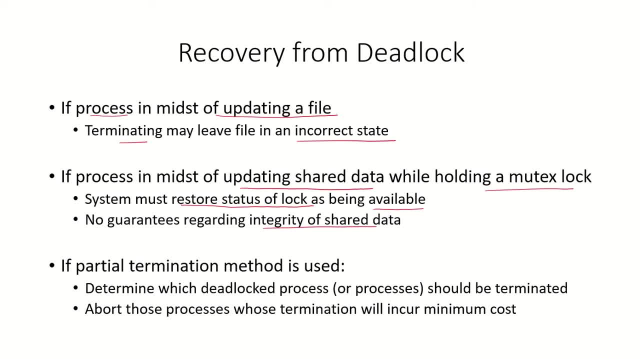 of updating this shared data. the process has now been aborted. Now, if we use the method of partial termination, that means we are terminating only one process at a time. So out of all the deadlocked processes, we have to determine that which deadlocked process should be terminated. 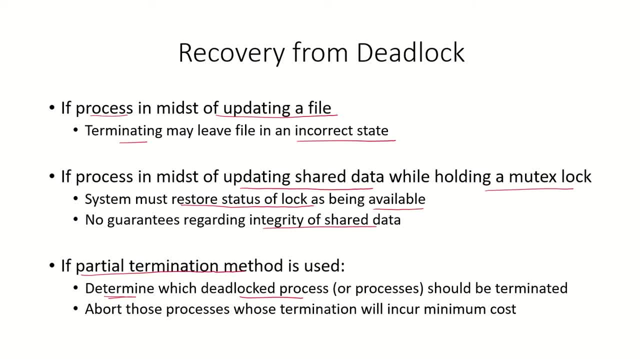 And the strategy would be to abort that process or those processes first whose termination will incur the minimum cost. So what do we understand from the cost? Because when we are terminating a process, there are various factors which are associated with it. That means how much computation? 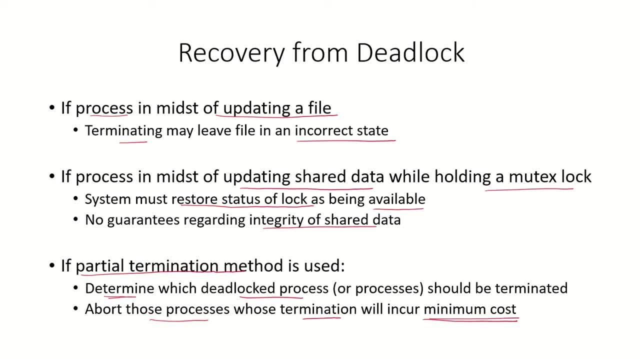 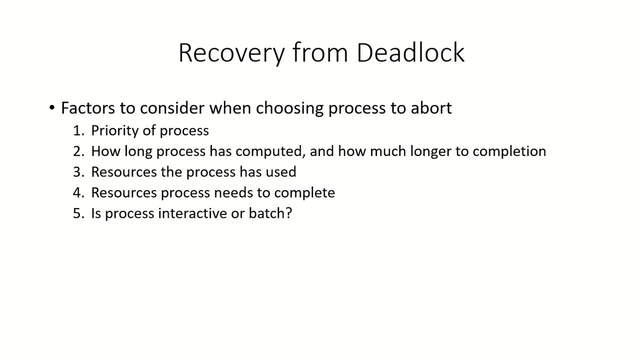 it had already done. what is the priority of that process? So, for with each process, there is some cost associated. So how do we choose which process will be terminated? So there are certain factors which we can consider and these can also contribute to the cost, and these 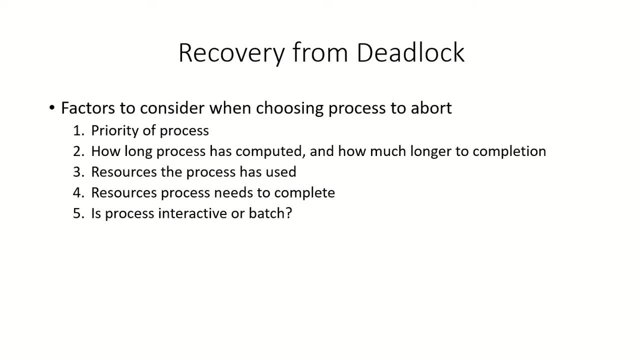 factors can help us decide which processes to abort. One is the priority of a process. So if there are three processes- P1,, P2, P3- and if the priority of process- let's say P3- is the highest, we would not want to terminate this process. P3 first, We will choose a lower. 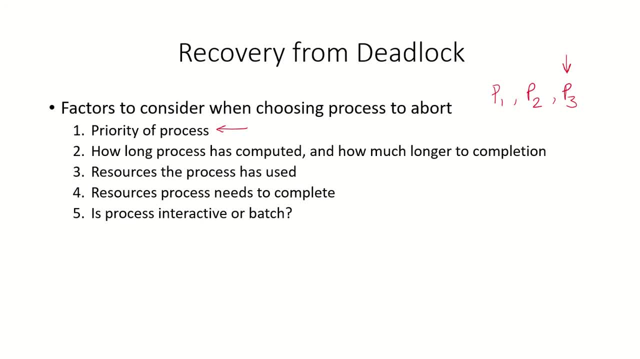 priority process. A second factor to consider is how long the process has computed and how much longer to completion. So let's say this has computed for ninety percent of the computations are over. This has done only thirty percent and this has done seventy percent, Then it would make 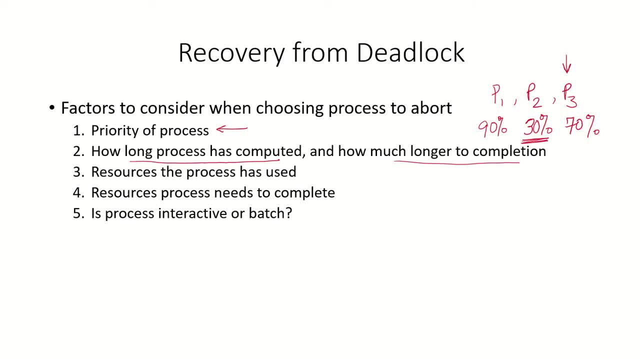 sense to choose process P2 because it has not computed as long as P1 and P3. So P2, since it has done less of computation right now and it will require longer to completion, then it makes sense to choose P2 for abortion. Then how many resources the process has used. 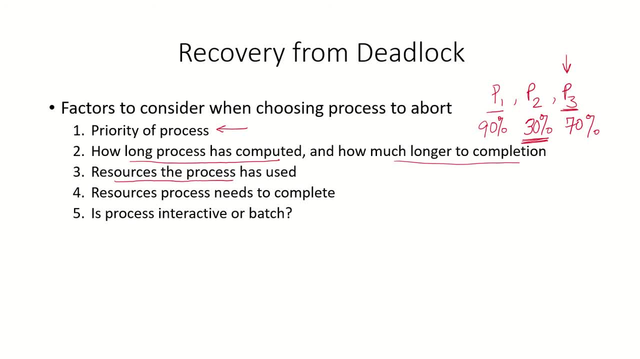 If a particular process is using more number of resources compared to other processes, then there is a possibility that that process can be terminated first so that it will release all those resources and those resources can be used by other processes for removal of this deadlock. Also, how many resources a process needs to complete. So if a process now requires 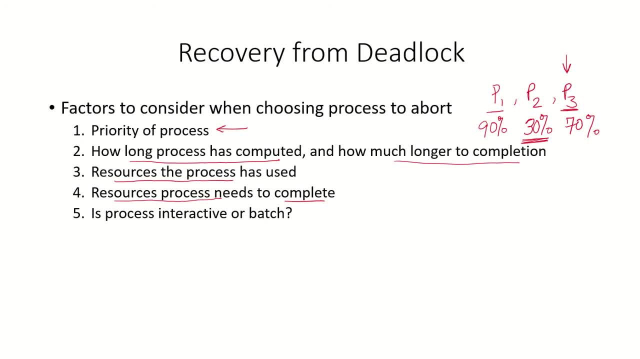 more number of resources. that process should be terminated first. Let's say, requires 10 resources, P2 requires 2 resources and P3 requires 5 resources. So since P2 is requiring less number of resources, it makes sense to let this process exist and terminate. 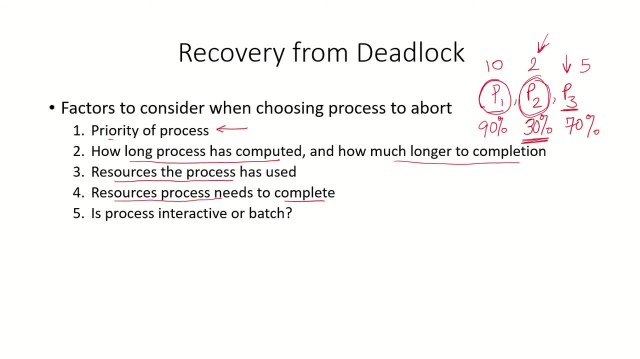 process P1.. So all of these factors, priority, how much it has computed, the resources it has used and the resources it needs, all these factors, they will contribute to choosing the process which has to be terminated. Another factor is: is the process interactive or a batch process? 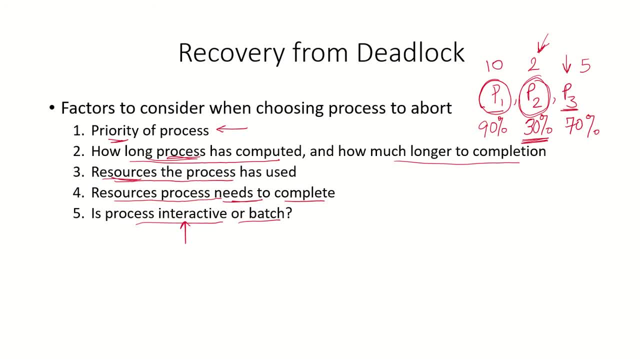 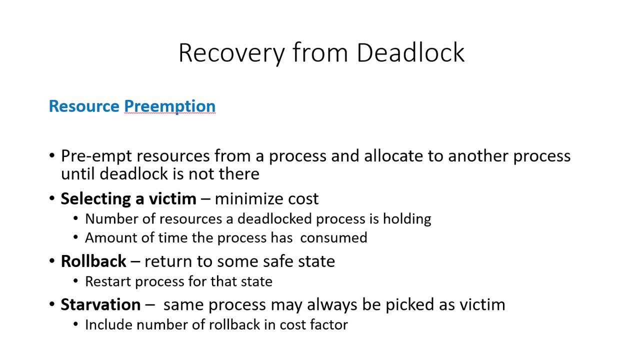 So if it is an interactive process, it will be given a higher priority and not be terminated compared to a batch. So rather than using this strategy of process termination, there is another strategy, which is resource preemption. Here we preempt resources from a process and allocate it to another process. 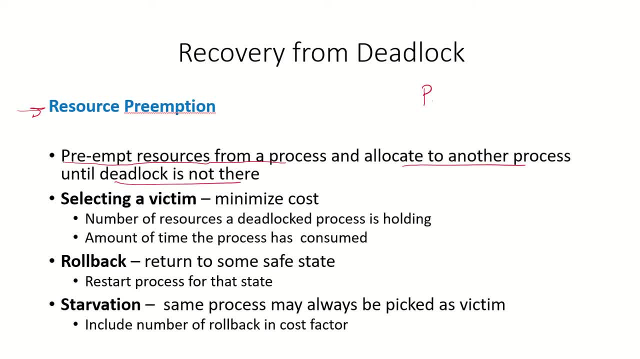 till the time the deadlock is not there. So we have, let us say, P1, P2 and P3, which are involved in a deadlock, and now what happens is we have a process termination, which is called a batch process. So what is going to be done is that, from a particular process, resources are going to be 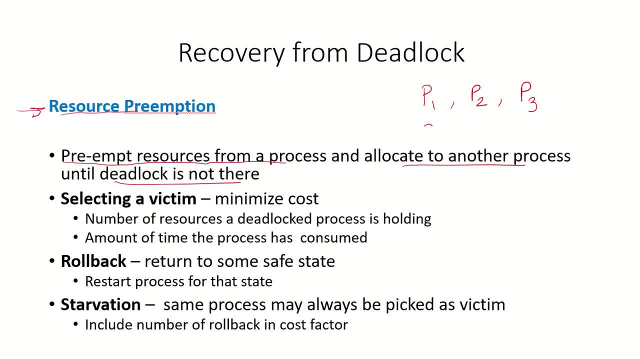 preempted. So let us say P1 is using 3 instances of one resource type and this is using 5 and this is using 7 and they are requiring more. So one of the processes will be preempted and its resources will be given to the other processes which are involved in the deadlock. So now how to select. 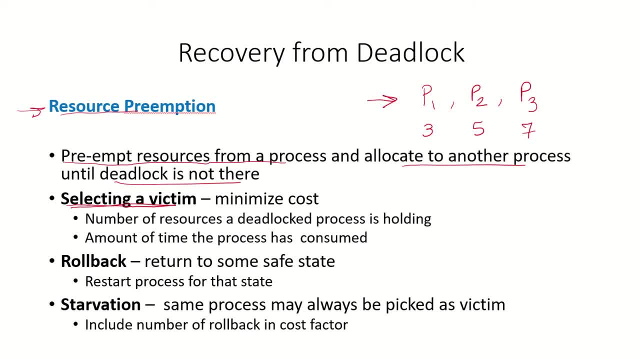 the victim? Now, out of these processes, which process should be the victim? That means from which process the resources should be preempted. Obviously, that process which will have the minimum cost associated with it will have to be chosen. and again to compute the cost, all these factors, 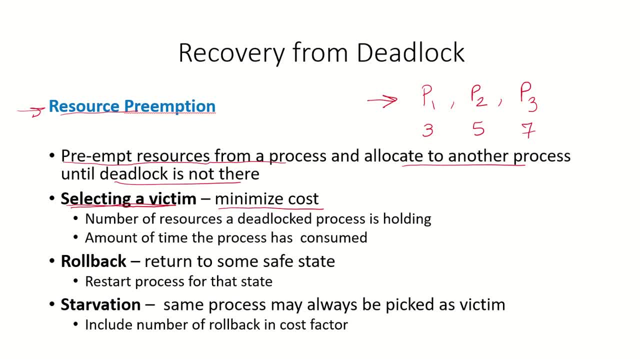 can be taken into account. So, whichever process is incurring the minimum cost, that will automatically be taken into account, and whatever process is incurring the minimum cost, that will also be taken be chosen and resources will be preempted from it. Now again, there is another possible thing. 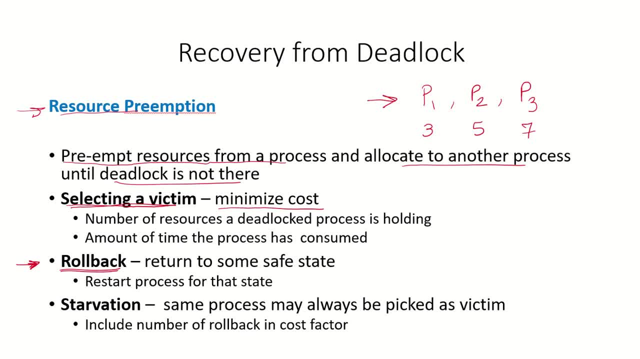 that we need to take care of is the rollback. So let us say resources have been preempted from process P3.. So if P3 resources have been preempted, that means now the process has to return to be to some previous safe state. Since this was already computing, it has reached a certain state. 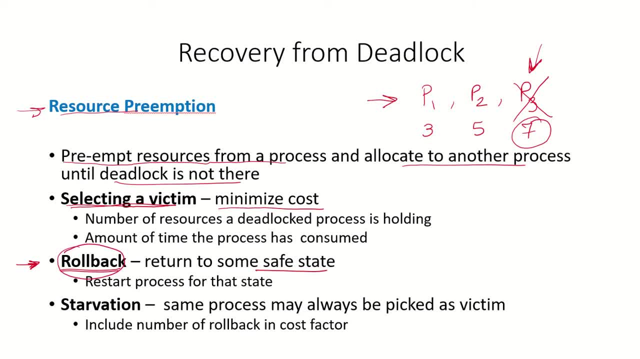 it has to be rolled back now to some previous safe state and then whenever it starts computation next, it will start from that particular state. Now, when we do this resource preemption, there is a possibility that the same process may be reelected from P3. So if P3 resources have been 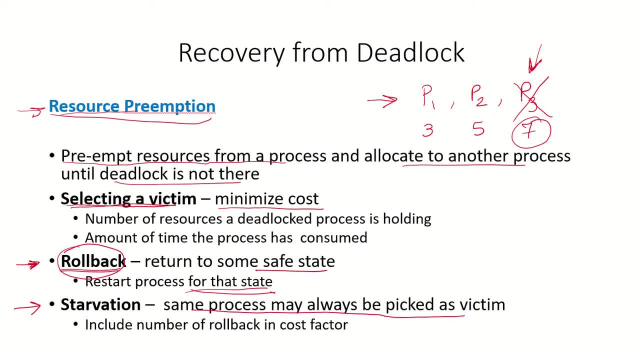 preempted from process. P1, P2, P3 may always be picked up as a victim. Now let us say P1 and P2 and P3 were in a deadlock and P3 was chosen as a victim process and its resources were preempted. 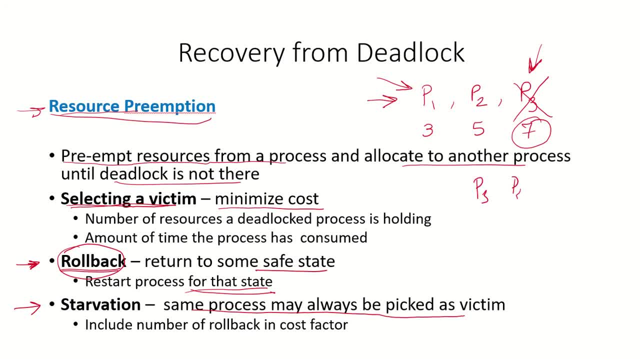 After some time, let us say, P3, P4 and P5 are in a deadlock and again P3 is chosen to be the victim process and its resources are preempted again and given to other process. So this is going to cause some starvation and then the process will be reelected from process P3. So 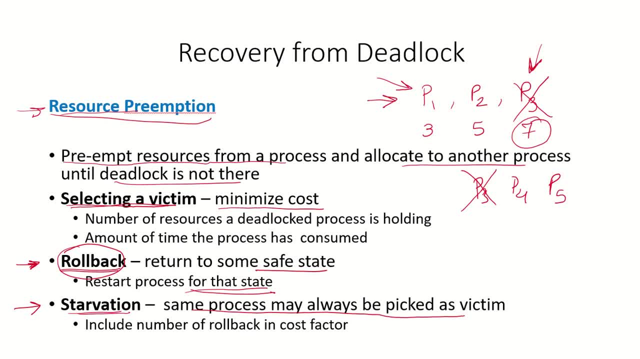 that means every time the same process is picked up as victim, it will not be able to execute, it will not be able to compute. so this should not be done, it should be avoided. so it's always a better idea to include the number of rollbacks also as the cost factor. so when we are considering all these, 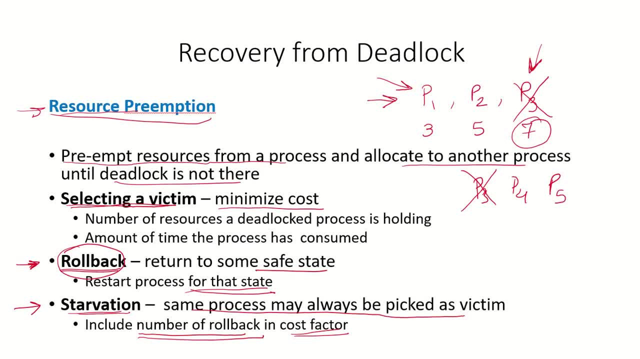 factors while computing the cost, then the number of times a process has been rolled back should also be considered. so if p3 has been rolled back once over here and another one over here, so the number of times this process is being rolled back should be considered as past part of the cost, and then the next time.